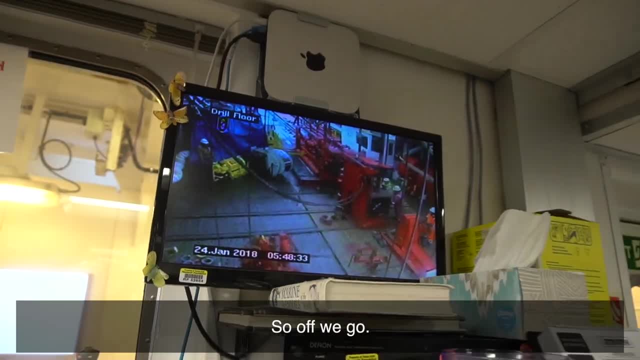 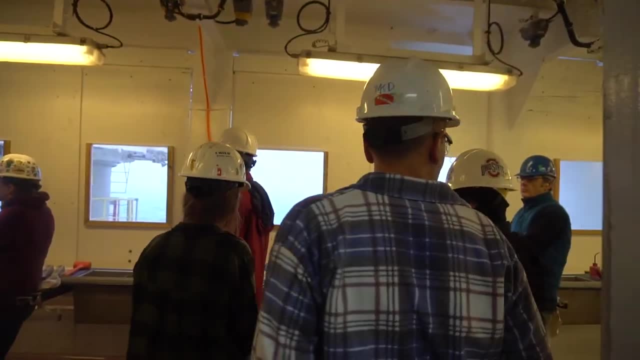 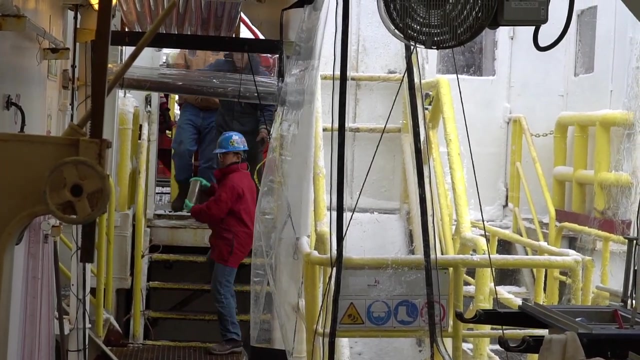 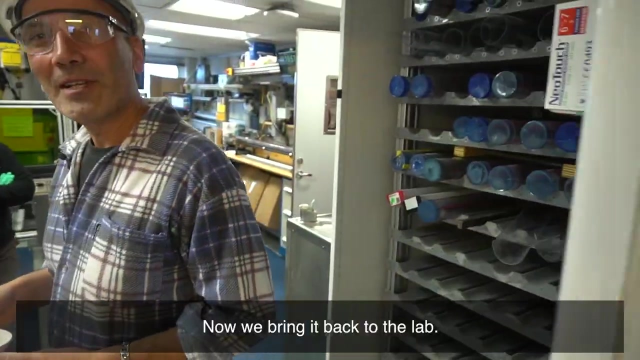 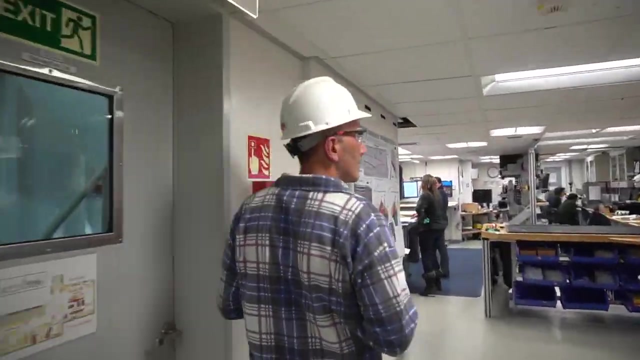 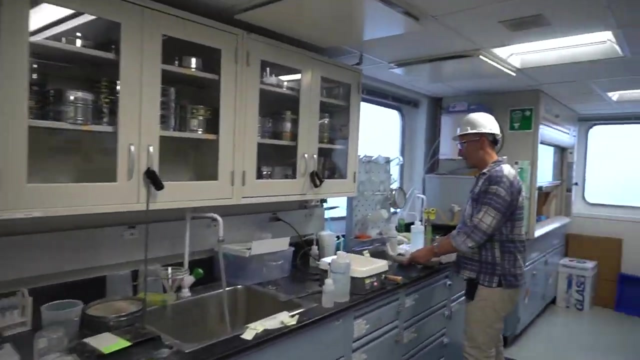 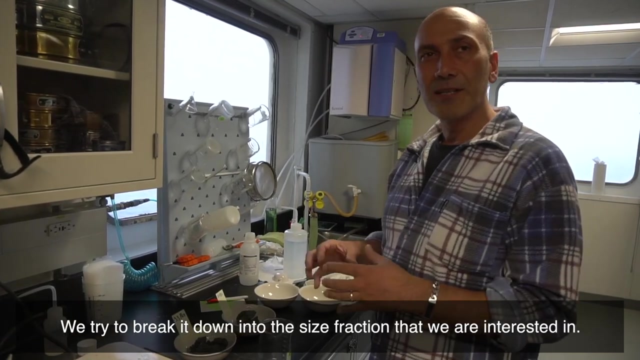 Cortex. Now we bring it back to the left, And this is the place where they live here. So it's all these little bowls, and we try to break it down in the size fraction that we are interested in, And then we put hydrogen peroxide. 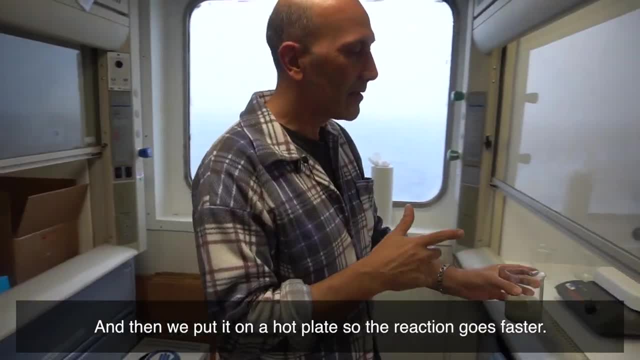 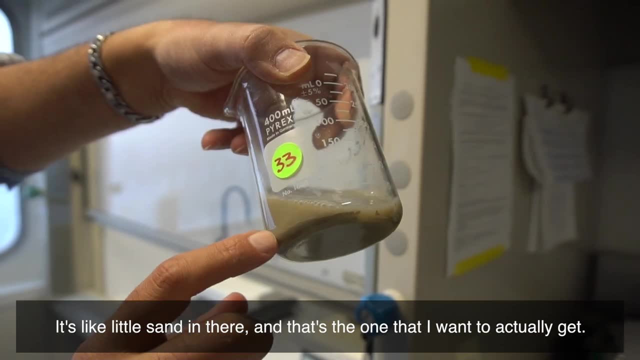 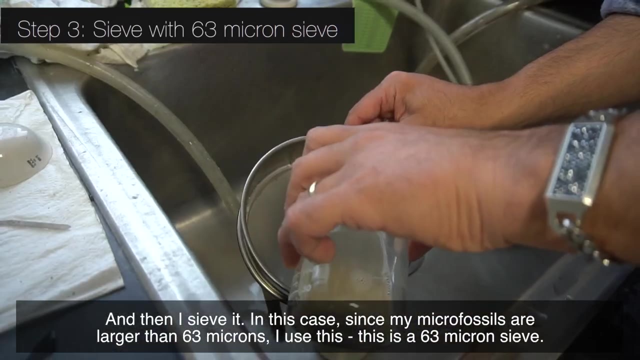 to dissolve the organic matter, And then we put it on a hot plate so that the reaction goes faster. Little sand in there, And that's the one that I want to actually get, And then I sieve it. I sieve it through. In this case, since my microfossils are larger than 63 microns, I use this. 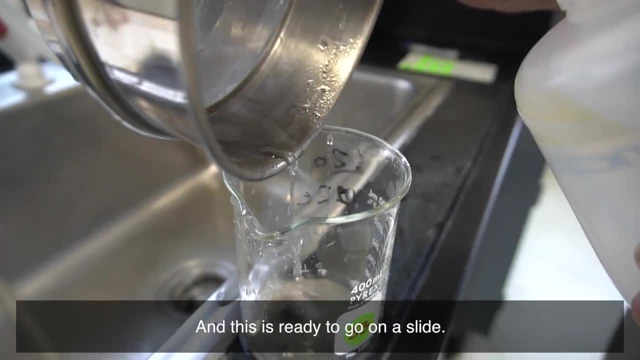 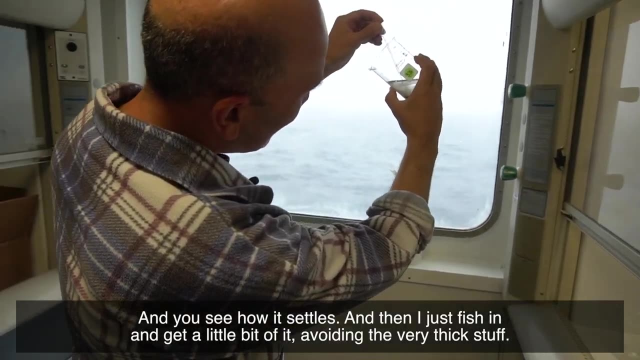 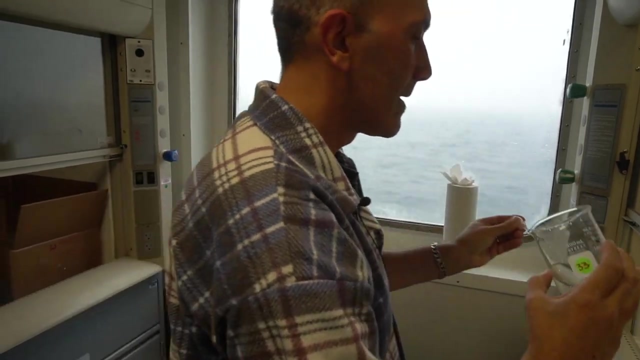 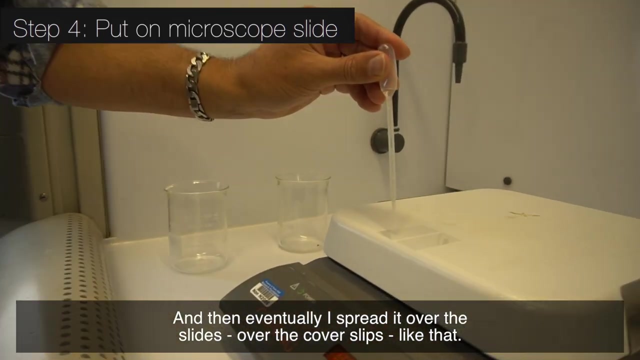 This is a 63 micron sieve And this is ready to go on a slide And you see how it settles And then I just fish in and get a little bit of it, avoiding the very thick stuff, And then eventually I spread it over the slides, over the coverslips, like that. 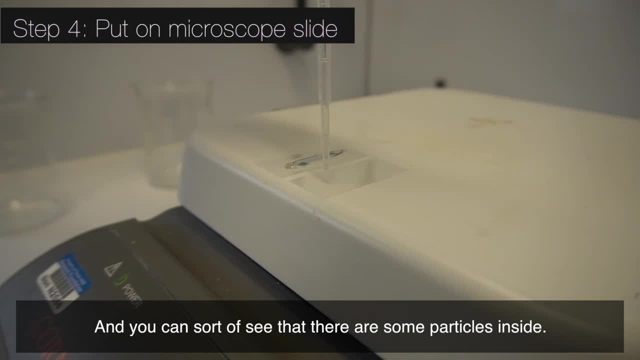 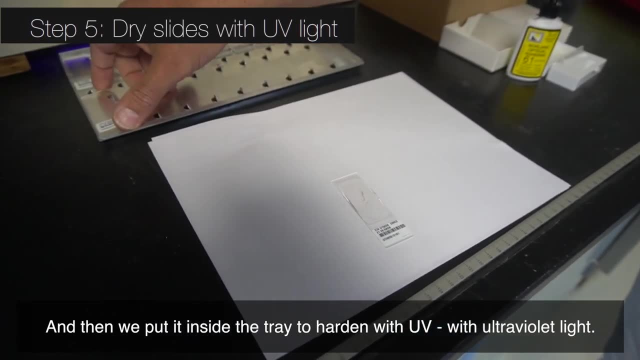 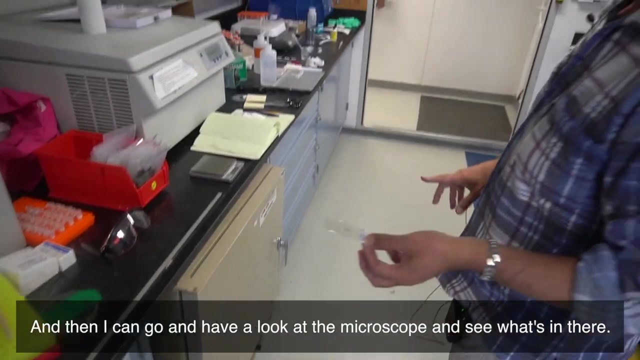 And you can sort of see that there are some particles inside, And then we put it inside the tray to harden with UV, with ultraviolet light. These slides are ready to be observed at the microscope And then I can go and have a look at the microscope and see what's in them. 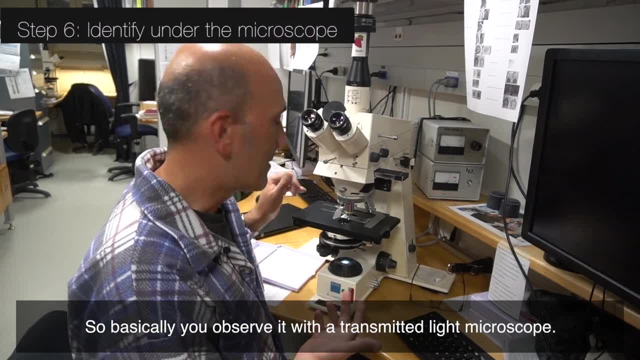 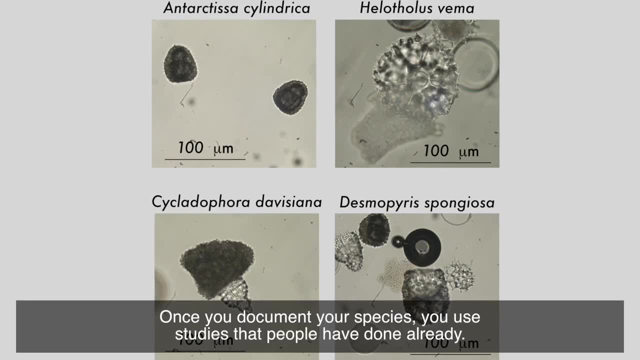 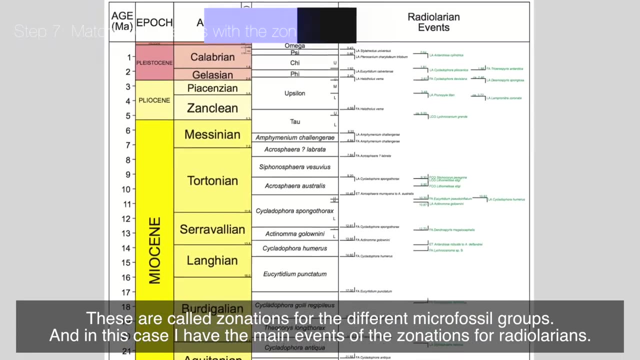 So basically, you observe it with the transmitted light microscope. Once you document your species, you use studies that people have done already. These are called zonations for different species. These are from macrofossil groups And in this case I have the main events of the zonations for radiolarians. 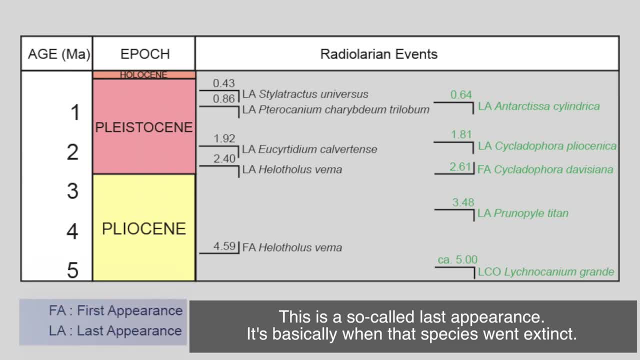 This is a so-called last appearance. It's basically when that species got extinct- And I have different species which have been recognized as actually appearing or disappearing at a specific level in time, And then people have calibrated that moment with paleomagnetism.